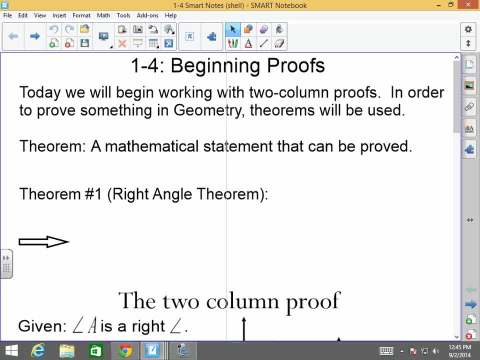 Because in another book maybe that's theorem 5.. Or in another book maybe that's theorem 3.. So saying theorem 1 isn't consistent mathematically throughout the world, But the right angle theorem, that's consistent Okay. 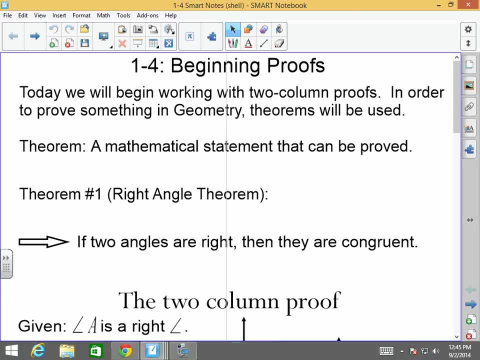 And what is the right angle theorem? Well, it's very simple. The right angle theorem states that if two angles are right angles, then they are congruent. It's literally that simple. If you see that two angles are right angles, then you know that those two angles have to be congruent. 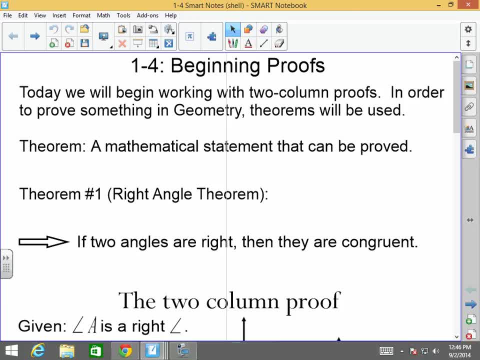 Why? Why? Because right angles mean that they have 90 degrees, And if you have two right angles, that means that you have two angles that are each 90 degrees. If you have two angles that are each 90 degrees, guess what? y'all. 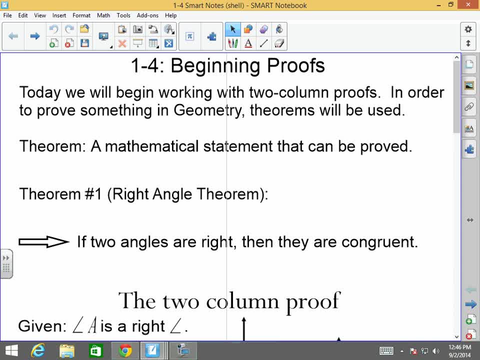 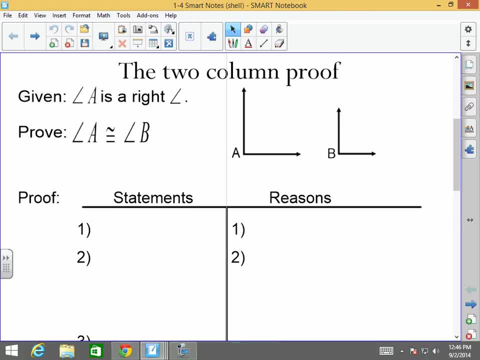 It is congruent. They are congruent, Okay. So let's start with a little proof as to how this is used. When you are going to be proving things. we're going to primarily use the two-column proof. We're going to learn later on this week that we can do something called a paragraph proof. 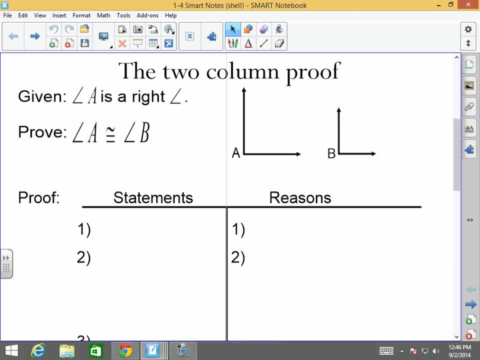 It's really up to you, but the two-column proof is more concise, it's quicker and it gets to the point immediately. Okay, So this is the way the proof is set up. before I even get into it, Notice how you have two columns here. 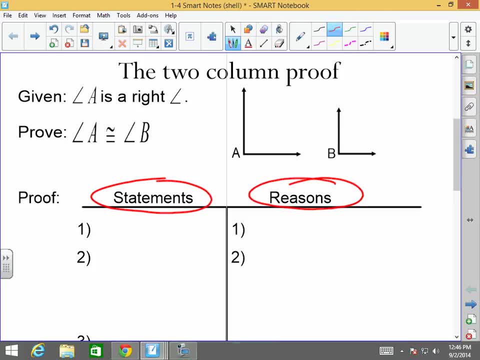 You have statements and you have reasons. You have reasons. You cannot put a statement down without a reason Why? Because that's just the way it goes in geometry. You cannot say, oh, because I think so Or because it looks like it. 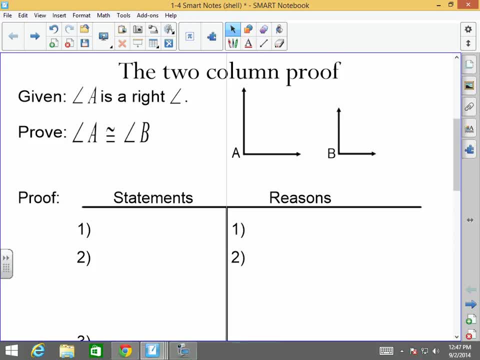 You have to be able to prove it. So let's get right to it. In any proof, they are going to give you a given and then something that says: prove Sometimes, Sometimes, Sometimes, Sometimes, Sometimes, Sometimes, Sometimes. 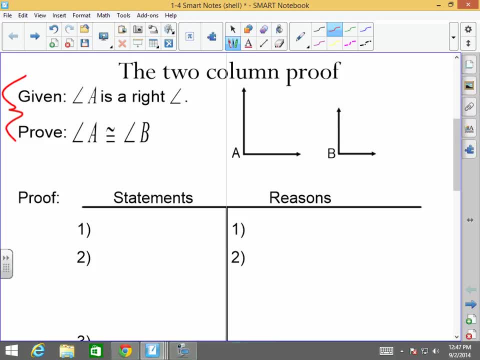 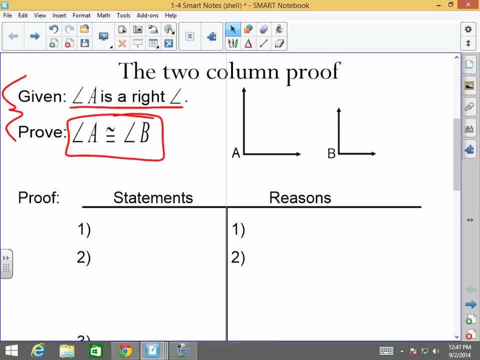 So first thing you're always going to do, no matter what: if you can do this, you're going to get at least a few points on the proof. I promise. Write down the given information And from the given information, then proceed to see what other theorems 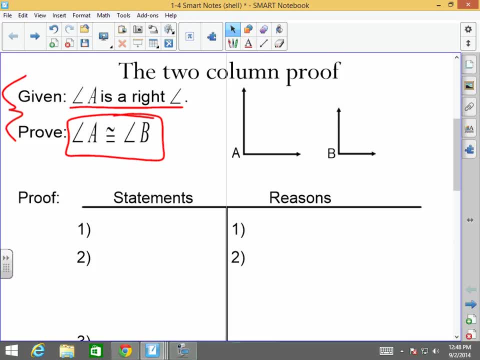 or definition or postulate I can use to continue my proof. So here, the given is that angle A is a right angle. Okay, Angle A is a right angle, And I forgot another given. The second given- I apologize- is that angle B is a right angle. 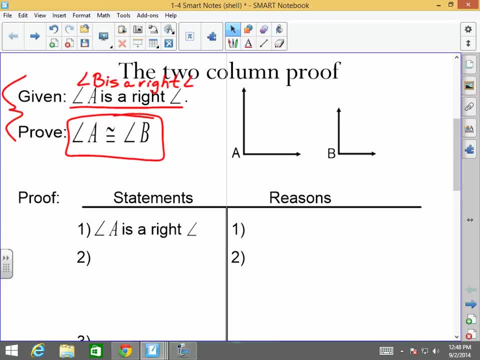 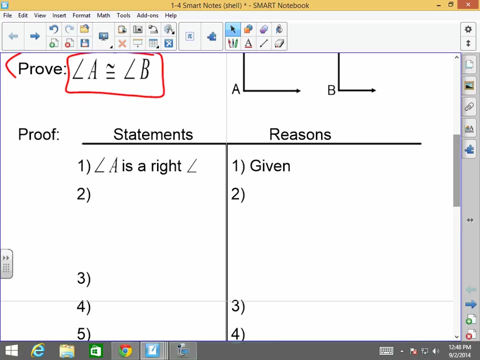 I got to make that, make a little typo here, So sorry about that. Okay, So if angle A is a right angle, why? Because it was given Literally. They gave you that information. Now, from here, what do we know about right angles, guys? 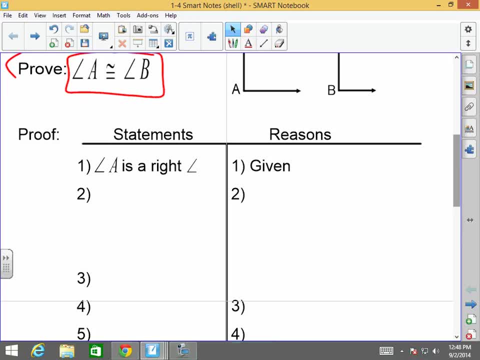 They're 90 degrees. So, guess what? Follow the pattern of thought. Since angle A is a right angle, that was given, I know, for a fact. we already learned the definition of right angles And the measure of angle A then has to be 90.. 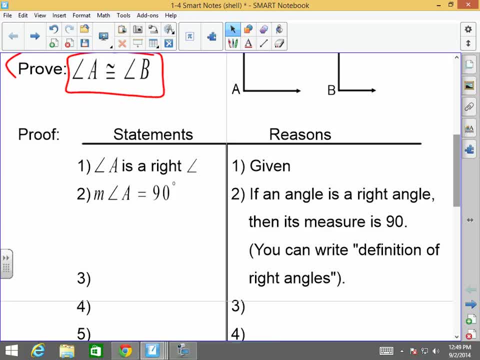 Why, If an angle is a right angle, then its measure is 90 degrees. I am not a stickler for Having to explain every theorem word for word. I am a stickler, though, for you understanding the concept. So, if you really think about it, we already defined right angles as angles that have 90 degrees. 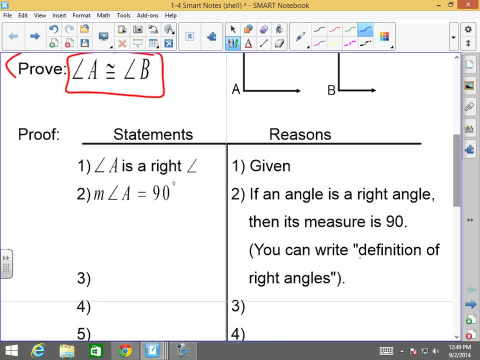 So you can write definition of right angles, Because already everyone in this class hopefully knows the definition of a right angle means that it's 90 degrees, So you don't have to write every time. If an angle is a right angle, then it measures 90.. 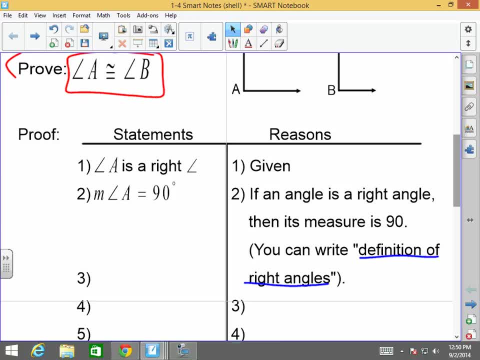 If you like that awesome Cool, Go for it, But you can write, in this particular case, definition of a right angle, If anyone is confused. again, why? Why could you do that, Mr Warren? Because you know the definition of right angles. 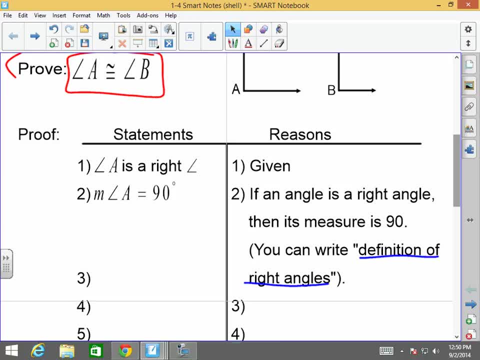 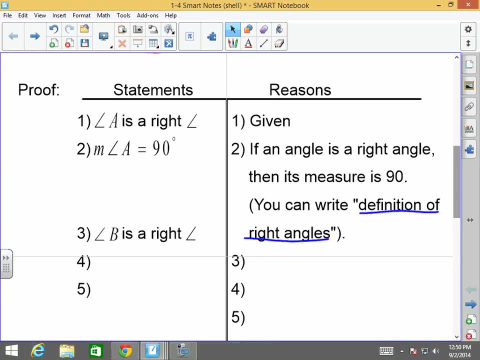 The definition of a right angle is an angle that measures 90.. Next step: That's about all I can take from the given information at this point. Step three: Angle B is a right angle. How do you know? Because it was given. 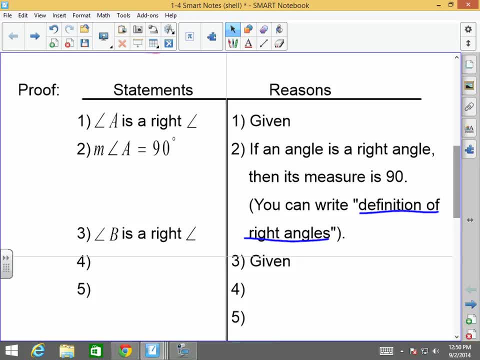 And if angle B is a right angle y'all, what do we know about the measure of angle B? then You're absolutely right. The measure of angle B equals 90 degrees, Why? Thank you, son. Definition of right angles. 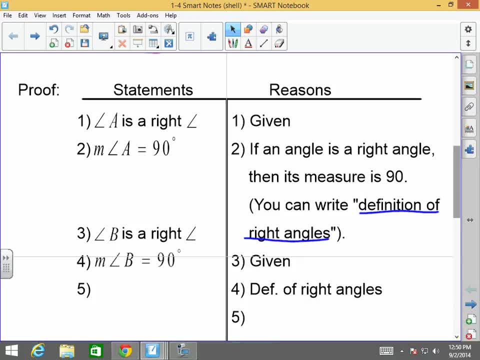 That's simple. Now that we have defined And proven That angle A is equal to 90 degrees and angle B is equal to 90 degrees, what can we say about two angles that have the same angle measure- That they're congruent? 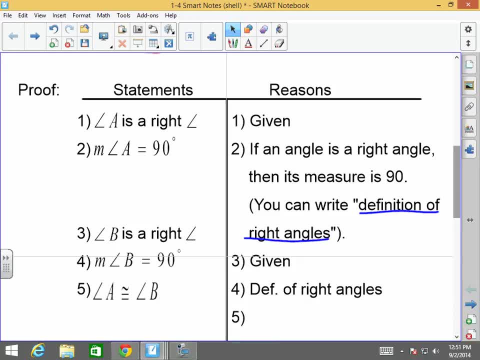 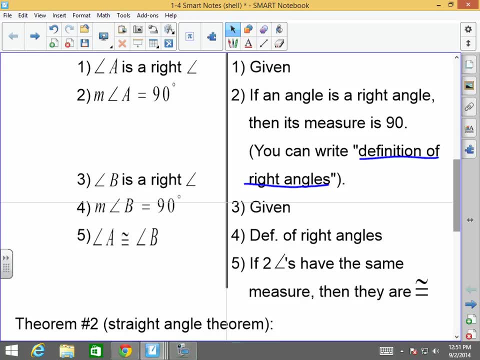 And guess what, my brothers? That's my proof. Angle A is congruent to angle B. Why? If two angles have the same measure, then they are congruent, And that's a proof, A proof. There's no question to any reader out there about that. 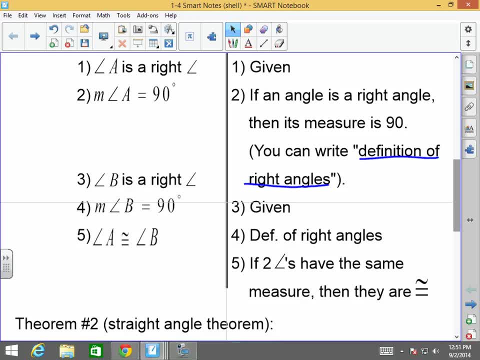 No one can argue that because it is proven. Does that make sense? y'all Awesome. Now theorem two. We're talking about the straight angle theorem. Now think about what we just defined as the right angle theorem. What would you think? 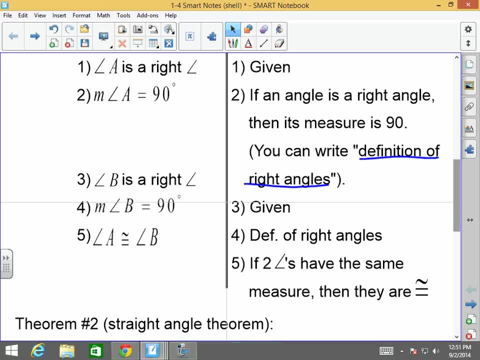 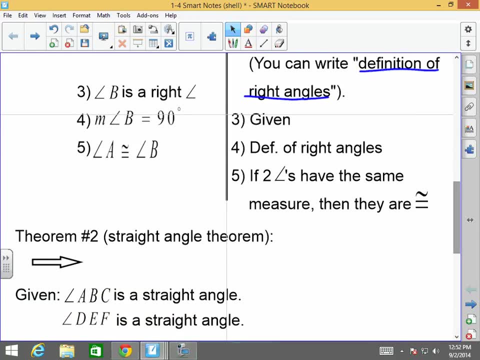 What do you think? the straight angle theorem states, guys, Any thoughts at all. There's no right or wrong answer. Well, there's a wrong answer. but anyone want to try? You are on fire, brother. Straight angle theorem is very simple, just like the right angle theorem. 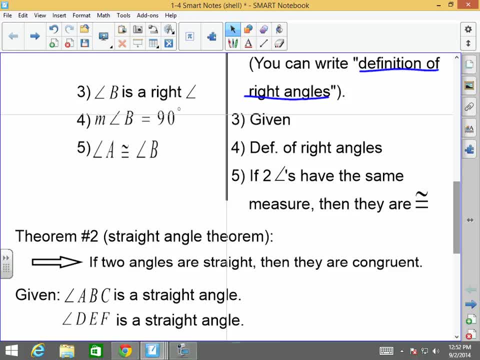 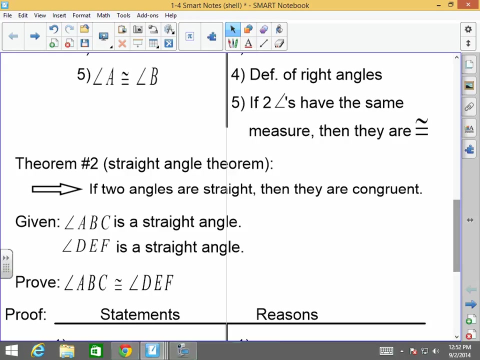 If two angles are straight angles, then they are congruent. Okay, if you wanted to, you can go ahead. um well, we'll get to it now in the proof. okay, two angles are straight angles, then they are congruent. make sense? okay, let's look at our next proof then. 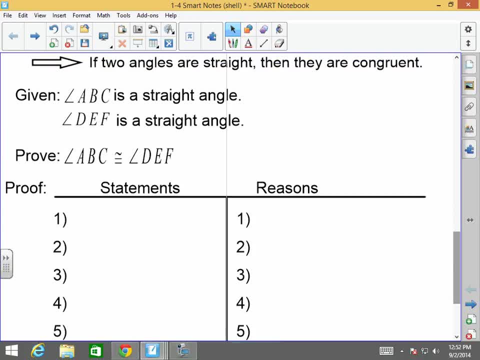 angle a, b, c is a right angle. an angle d- e is a straight angle. sorry, an angle d e, f is a straight angle. i want you to prove that a, b, c is congruent to angle d e, f. so sometimes they don't give you a. 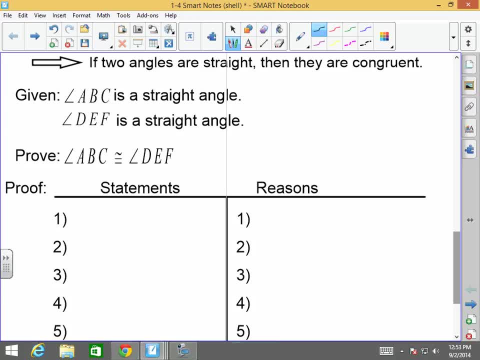 drawing. so make one angle: a b c is a straight angle. awesome, a b c, it's a straight angle. d e f is a straight angle. d e f is a straight angle. i want to prove, bless your son, that angle a b c is congruent to angle d e f. so we're going to orient it. 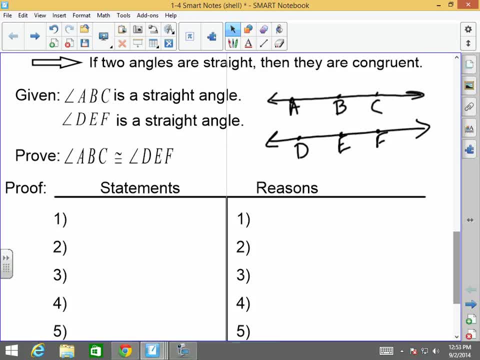 always start with our givens. Yes, sir, Correct, You're on fire. Angle ABC is a straight angle Reason given. What do we know about the definition of straight angles? Yes, sir, That is exactly correct. The measure of angle ABC then equals 180 degrees. Why, my brothers? Why? Thank? 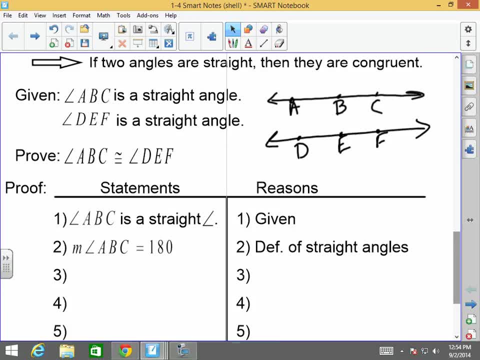 you Definition of a straight angle. Now, if you wanted to, you could say: if an angle is a straight angle, then its measure is 180 degrees. You can do that, but I'm not here to torture you. I want you to already know that definition. Oh yeah, straight angle. 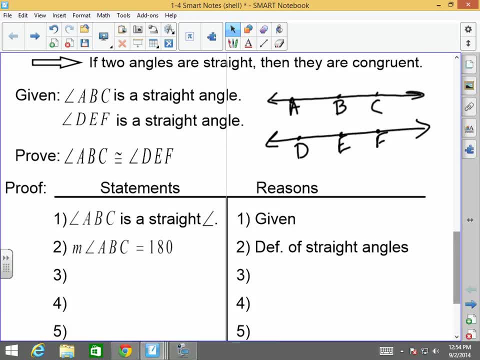 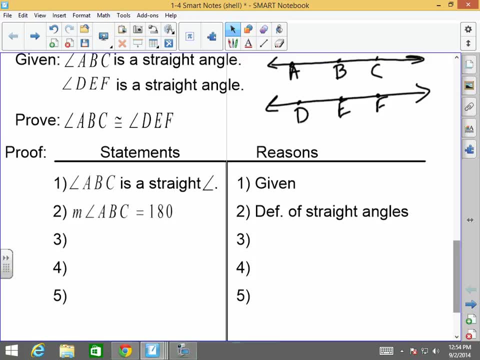 has to equal 180.. So the reason that angle ABC equals 180 degrees is because definition of straight angles. Number three: What do you think would be next? Sir, That's exactly correct. Angle DEF is a straight angle. Why It's given: Absolutely Always. write at least your givens. 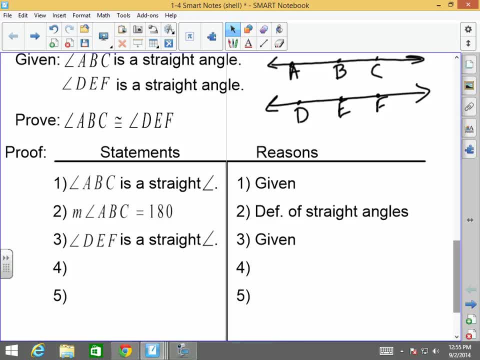 guys. Always, You're going to get some points at least that way. So if DEF is a straight angle, what do we know about the measure of angle DEF? Yes, sir, The measure. Yes sir, Always remember Great job, Always remember to put that little M. 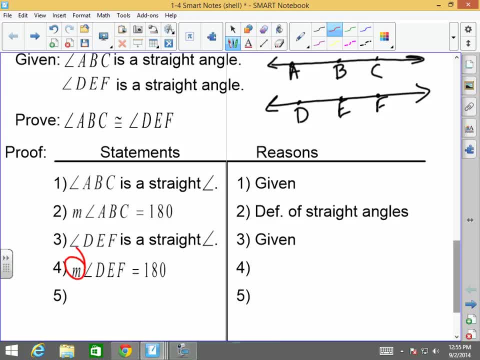 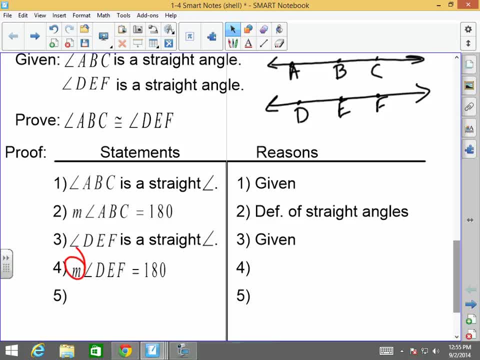 Okay, guys, I just want to give sign to you. Some people write all the givens first and then they expand upon it, but I find that sometimes that could be a little tedious, especially if you have 12,, 10, 15 different lines of proof. 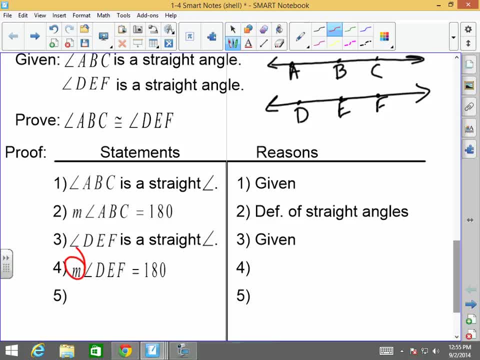 so what I always do is I always write my first given and I say to myself: okay, how does that information help me? How does knowing that angle ABC, for example, in this particular case, it help me? knowing that angle ABC is a straight angle? Well, the only thing. 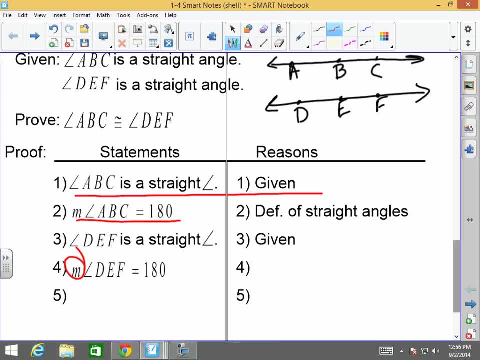 it tells me is that the measure of angle ABC is 180.. Now you're done with that given. Now you can move on. So there's different schools of thought. Some people write all the givens down immediately. You can. There's nothing mathematically wrong about. 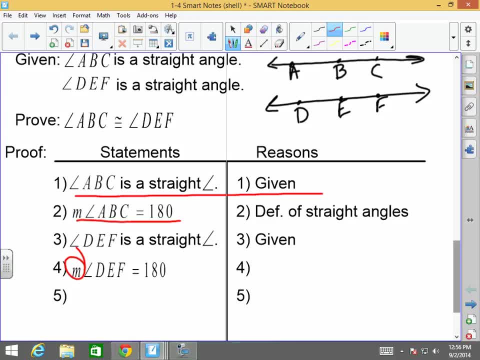 that. However, logically speaking, the whole point is to have a given Okay. how can that help me? What does that tell me? What does that give me? Have a given Okay, how does that help me? What does that tell me? 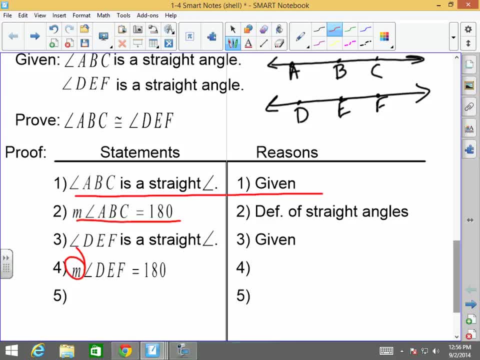 Thank you very much. Now the measure of DEF is 180.. Why Definition of straight angles, Sir Sure? and then what's number five? my man, You're almost on. No, no, no, no, You're right, I'm going to let you continue. 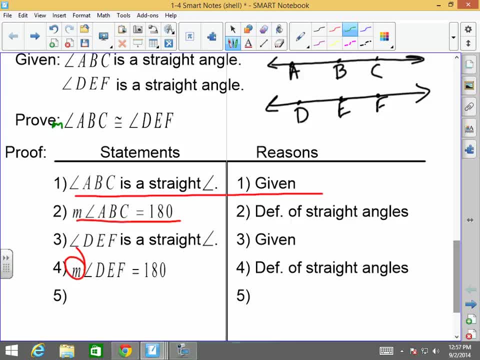 The only thing you had said my man is. you said measure of angle ABD and measure of angle DEF. The measure was given here. Okay, we did these two measurements in order to prove congruency. We know that 180 is equal to 180.. 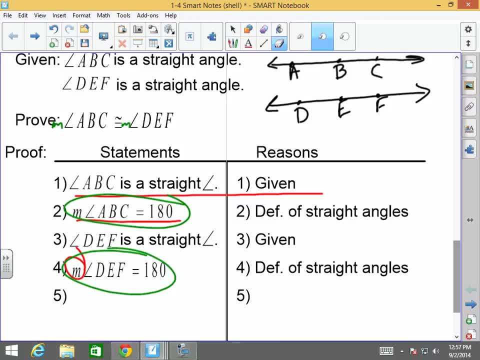 But at the end they're not asking if the measure of the angles are congruent, just if they're congruent by them. So take off that measurement part and then repeat what you were going to say. my man, That's what I'm. 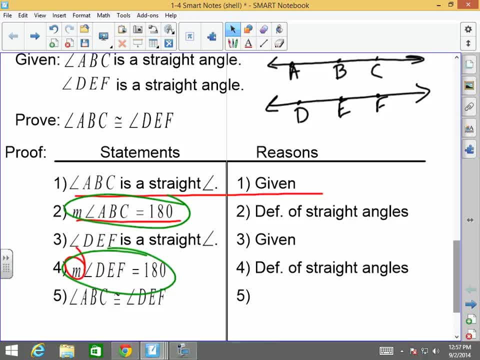 talking about, because that's what I'm trying to prove. Angle ABC is congruent to angle DEF. Excellent, Why my brother? Absolutely brother. If two angles have the same measure, they are congruent. Notice how I do a little shorthand. I try to do shorthand as much as possible. 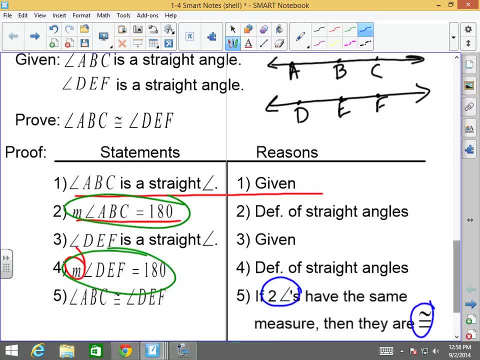 saves time, Do it as well. That is totally cool with me, Totally fine. Does that make sense? so far, guys, Right. Pretty easy, so far, right. All right, Let's do some sample problems with these two theorems. 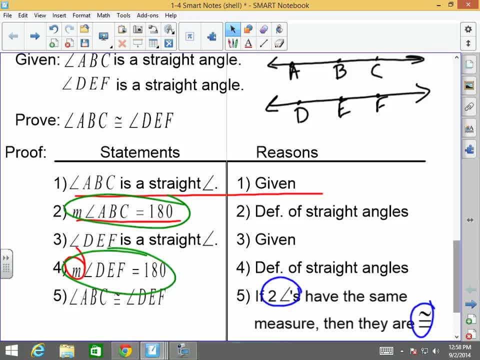 The good thing about this is we start slowly and we build. okay, It's kind of like a snowball. It just starts real small, but at the end of the year you're going to have this enormous amount of information, this huge pool of information. 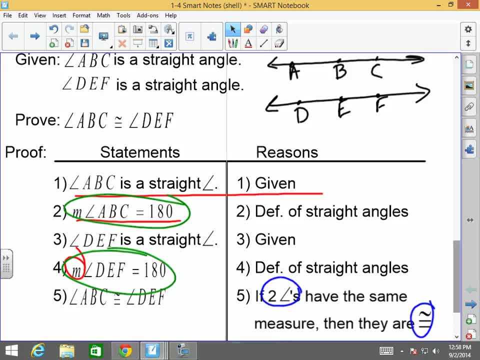 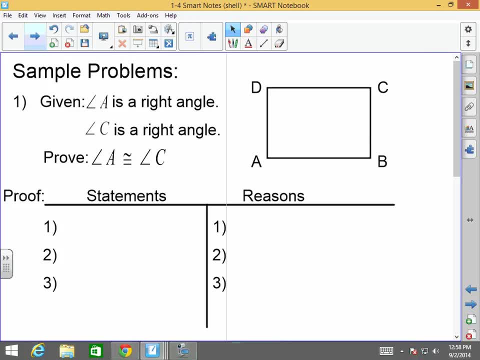 that you can just take stuff from and prove just about anything geometrically. May I continue? Thank you, Okay, boys. Given angle A is a right angle, angle C is a right angle. Prove that angle A is congruent to angle C and they give us this figure, okay. 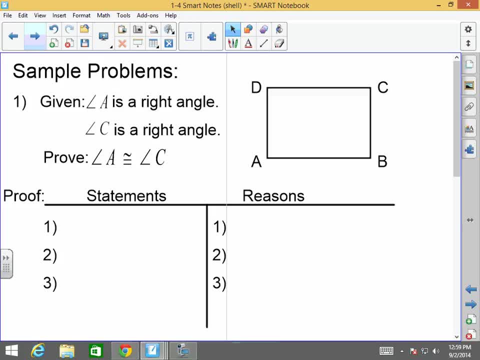 One thing that I always like to do is I always like to use the drawing to my advantage. So immediately I always say to myself: okay, wait, A is a right angle, C is a right angle, It's visual. Now I know what I'm. 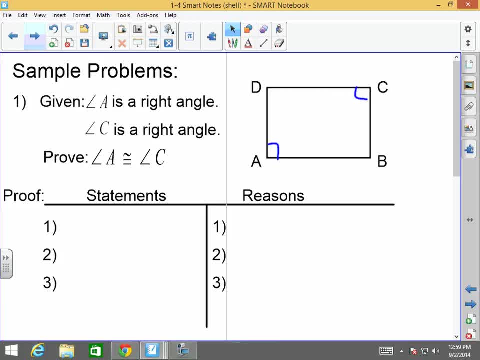 talking about Now. my goal is to prove that these two right angles are congruent. So let's knock it out. What's the first thing I'm going to put down? Yes, sir, That's exactly correct, Correct. What else can I say Then? the measure of angle A is 90 degrees. Okay. 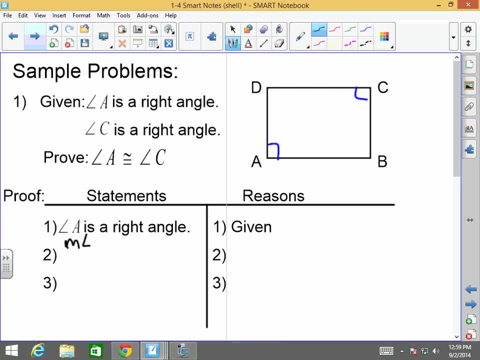 You're going to go above and beyond. I like that Measure of angle A equals 90 degrees. Yeah, So let's go ahead and change these numbers here, because you added a little bit more and that's fantastic. And then definition of: 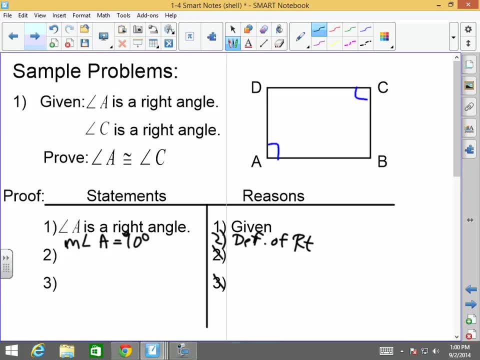 right angles Correct. Excellent, Next, Yup, And then That's exactly correct. Or definition of right angles Correct. Yes, sir, Angle A is congruent to angle C. You can come teach the class. Excellent job, son. 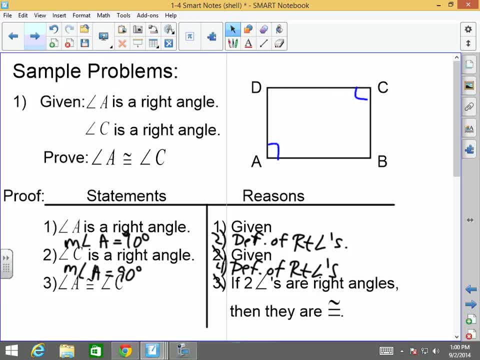 Very proud of you. Okay, Did that make sense there, guys? Now some of you may be saying, whoa, hold on, I'm a little confused, though. Mauro. My boy just gave us five reasons. Why didn't you include those reasons in there, Mr Mauro? Okay, 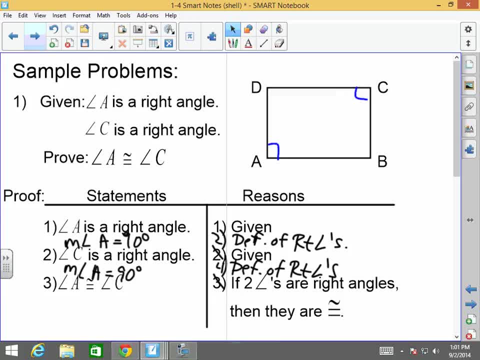 And our first proof that we did. we went real basic, But you know already that right angles equal 90 degrees, regardless, correct? And you know that if two angles are right angles, they are congruent, right. So you could go either route. here He went above and beyond. Not only did he, 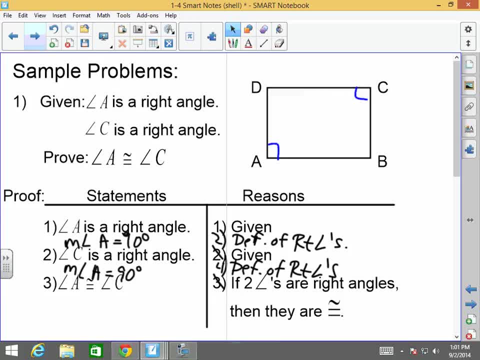 put the givens. he explained what the givens were and then he said: okay, two right angles must be equal. Okay, so you have a little bit of play here. There's not an exact science. for the most part, It's all. 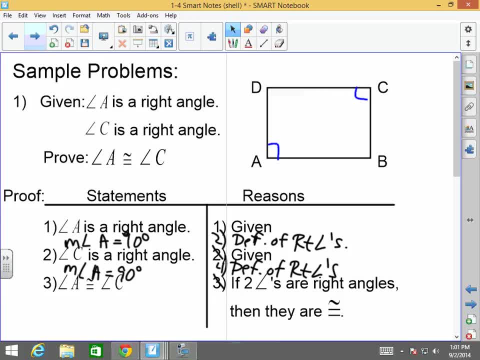 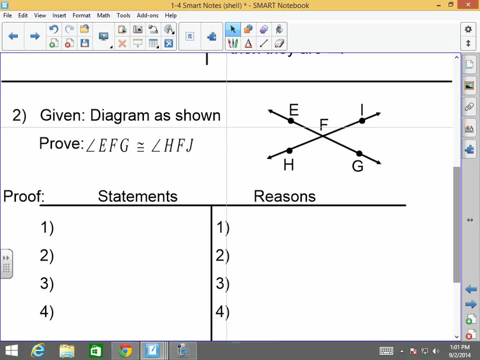 about how your mind is thinking, how it's bringing that information together. Cool, Alright, May I continue? Alright, And this diagram here, or the given in this case, is diagram as shown. Ooh, diagram as shown. What is that? 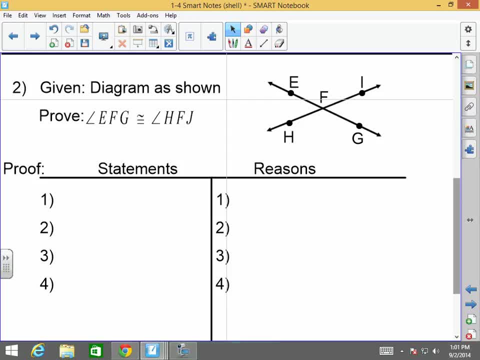 What can we get from here? Yes, sir, Yes, thank you, sir. That should be J. Yes, Thank you, son, That's exactly correct. But before we can assume those two things, we've got to use our given. 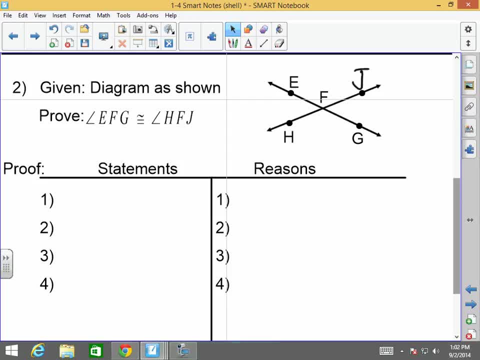 Because the given is letting the reader know: hey look, I took what you gave me and I'm putting it right here Now. from that I'm going to extrapolate all this information. So, diagram as shown would really be your first line of defense. 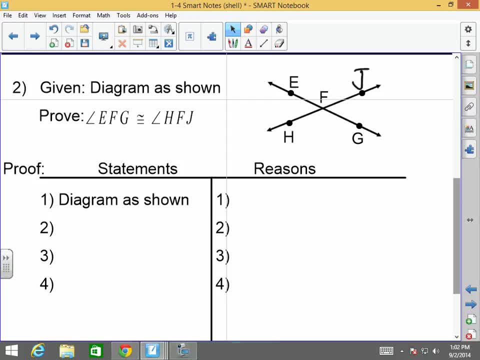 Why diagram as shown? Because that's what they gave you. It's given y'all It's given. Okay, Now angle two. exactly what my boy said: EFG is a straight angle. What's the reason, though? You had said it before. 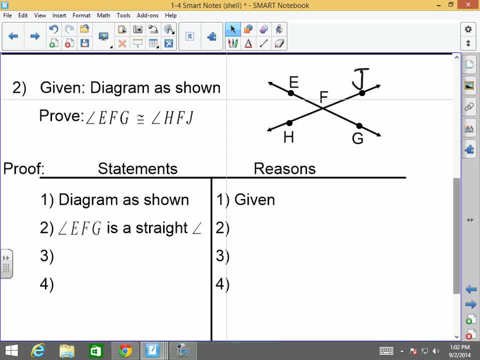 Yes, You can assume that. So you put: assume from diagram. Remember that you can assume straight angles. You cannot assume right angles, But you can assume straight angles. Next, on the totem pole, HFJ is a straight angle. How do we know? 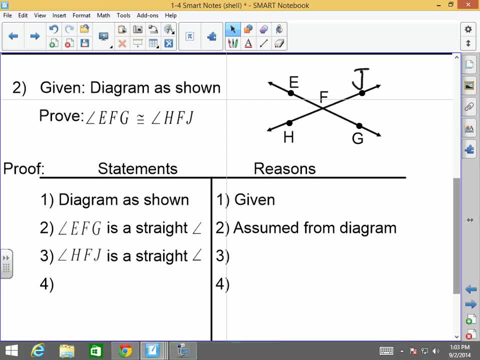 it's a straight angle, Because you couldn't assume it. Now, if you wanted to go above and beyond, you could say: the measure of angle EFG is 180,. definition of straight angle: The measure of angle HFJ is 180,. 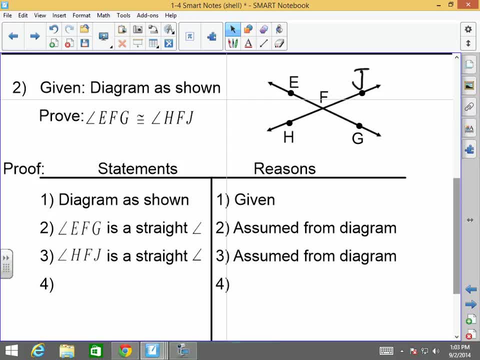 definition of straight angle. And then you can get to: if two angles have the same measure, they are congruent, Or we can just use theorem number two. And what does theorem number two state? Why is EFJ congruent to HFJ? 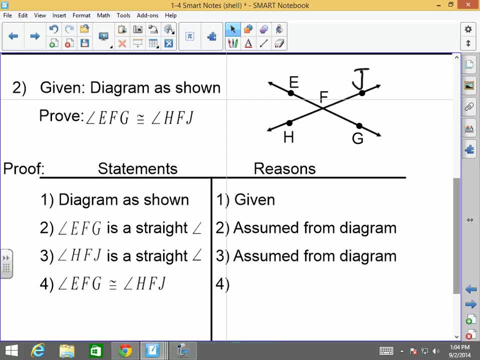 I mean EFG- congruent to HFJ. Why Use theorem two? Use theorem two, Bam. If two angles are straight angles, then they are congruent. Notice real quick the difference, though, guys. I don't want you to get confused. Let me split this in two. 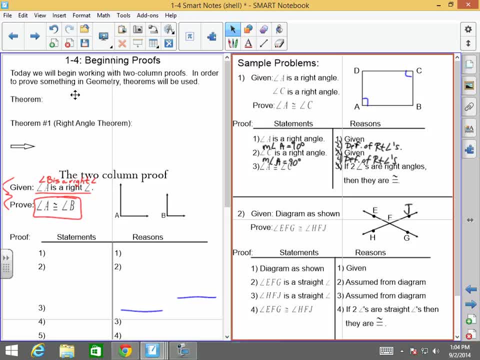 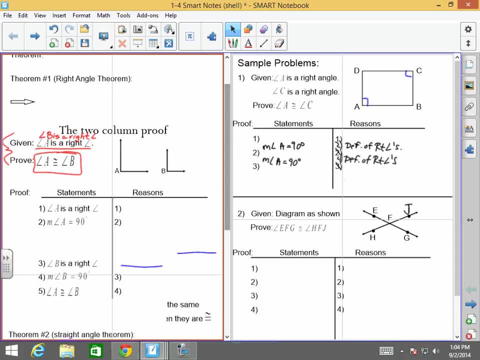 screens right quick. For this one we did not use if two angles are right angles, did we Here? we used a different proof Here. I decided to define my right angles by angle measures, so that I can say, hey, if two angles have the same measure. 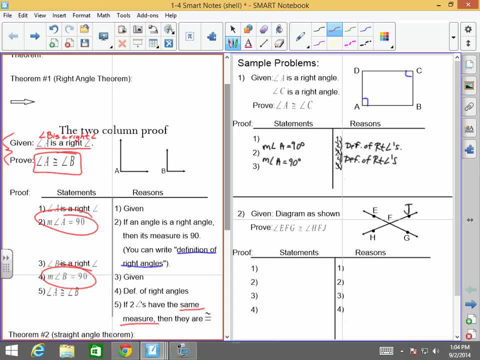 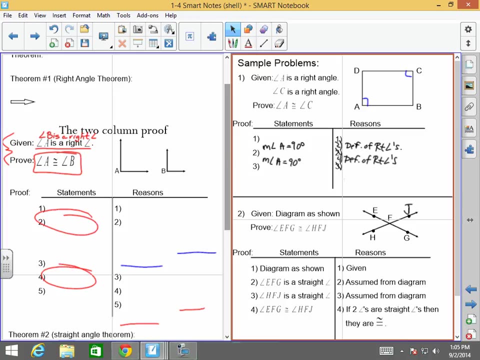 then they are congruent. But if I've already defined that they're right angles, or I've already defined that they're straight angles, that is why I am allowed to just go straight to the point. They're both straight angles, because I assume them from the diagram. and oh, wait a second, that's right. theorem two: 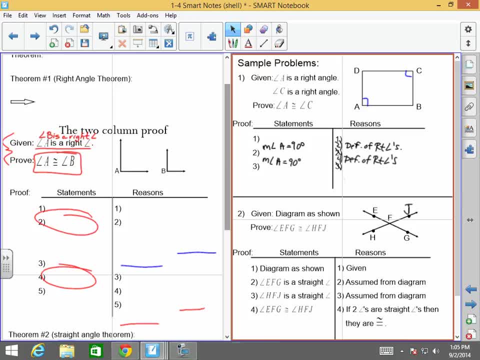 If two angles are straight angles, they're congruent. Boom, You don't have to prove their measure, Because you've already defined that they are straight angles, And if they're straight angles, they're congruent. Does that make sense? 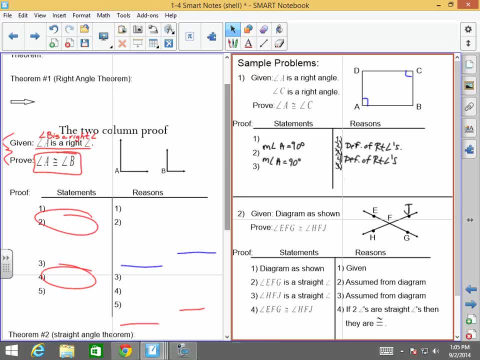 Especially for you, my brother, because you've been so detailed. Does that make sense? the difference of why I would put the measure and why I wouldn't? Thank you, Sir, Because that was my given. You always write the given. You always write the given. 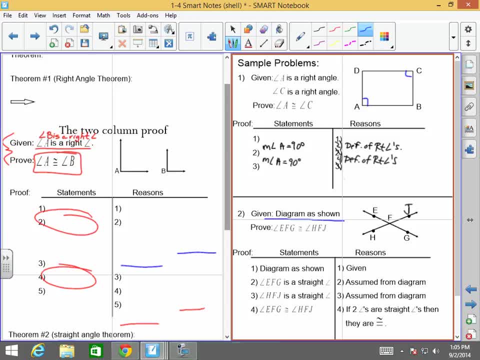 As the first one, Yes sir. And then figure out: okay, what can I extrapolate from there? What can I do from there now? Yes sir, go ahead, This is your class. Okay, Thank you. All right, This is. 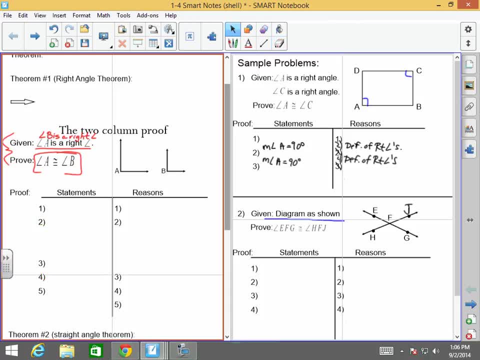 excellent, and this is exactly what I hoped for. Thank you so much. We're going to. I blanked it out. We're going to do it one more time. I'm going to use two different, two different proofs here. okay, And this first proof I wanted. 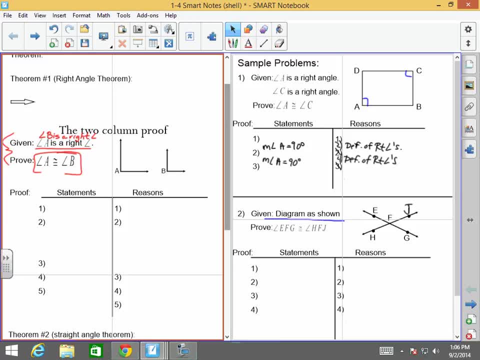 to prove that angle A is congruent to angle B. According to this, I know that angle A is a right angle and angle B is a right angle. So I want it to be a right angle, given a measure of angle A is 90.. If an angle is a right angle, then it has a measure of 90 degrees. 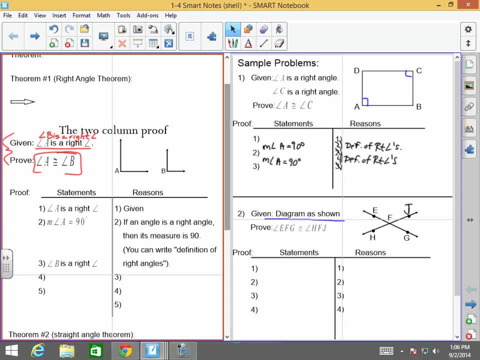 the definition of right angles. Angle B is a right angle, given the measure of angle B is 90 degrees. definition of right angles. Now we've already learned, before we started doing proofs, that if two angles have the same measure, then they are congruent. 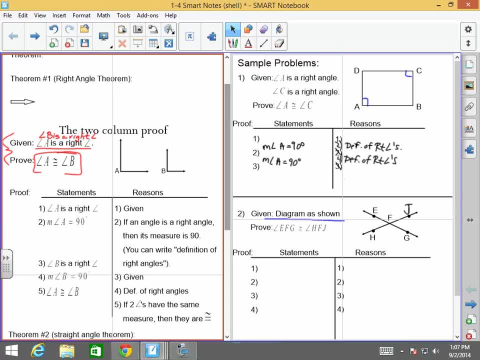 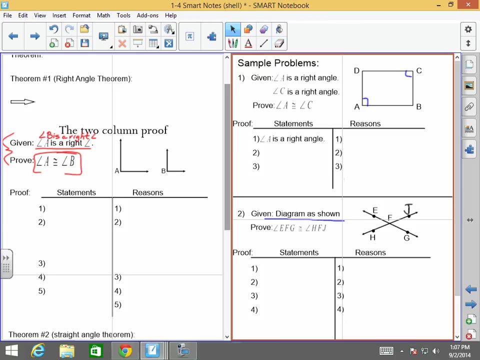 correct. Well, boom, That's what I did. However, we can condense this, though now using our theorems. For example, let's look at the sample problem number one. We said that angle A is a right angle given. angle C is a right angle given. 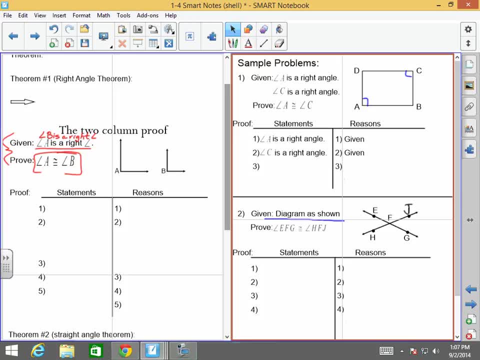 We don't need the measure now. Can you go the measure route? Yes, You can say that both of those are 90 degrees and that angles with the same measure are congruent, Or you could just realize: wait a second, I just learned a very powerful 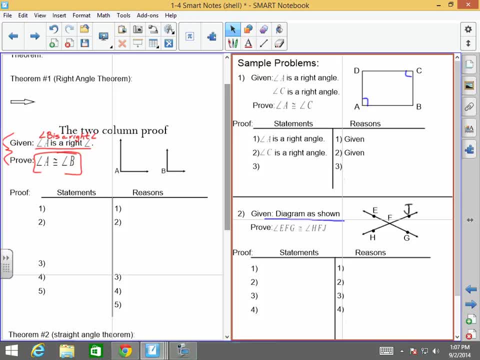 theorem. If I know that two angles are right angles, they are congruent. Why? Because if two angles are right angles, they are congruent. That's the theorem. Does that help you, sir? Thank you, Sir. Okay, the question was: can you just write down right angle theorem? 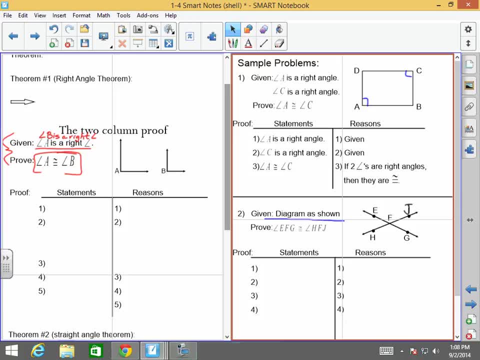 or do you write down the definition? Well, it really depends on a lot of things. I guess you could say right angle theorem. Yes, I would allow that. Yes, sir, I will allow that. Now, here's the only problem You're going to have: about 150 to 180. 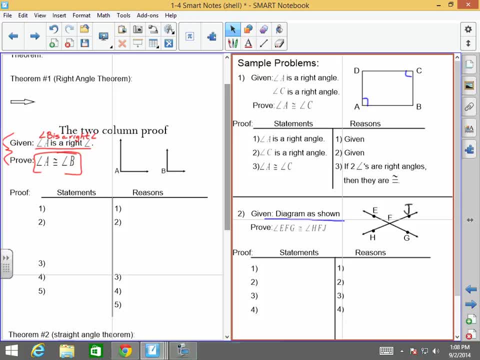 of these, So the name isn't going to always fly. So, just for building your confidence in this and building your strength in this, go ahead and define exactly what you're talking about. Define that theorem, okay. And then for number two, same. 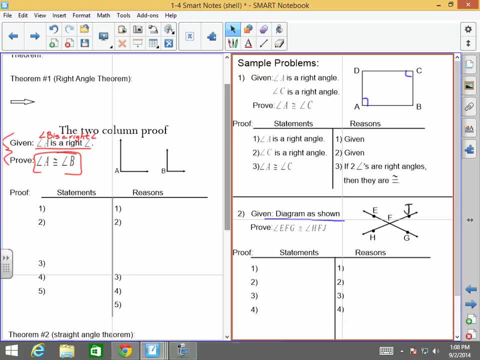 concept. We're going to prove this using a theorem, A new theorem that we learned: Diagram as shown. Okay, that's given. What can we tell from this diagram? Angle EFG is a straight angle, because I can assume that It's legal mathematically. 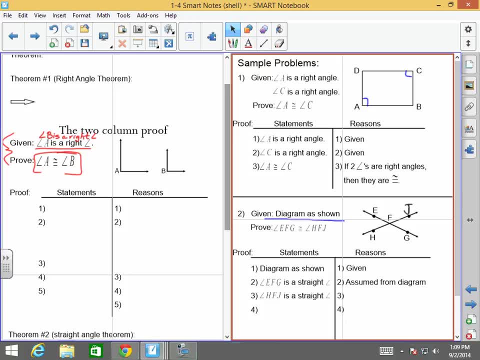 speaking Number three: HFJ is a straight angle. That's assumed. Wait a second. I don't have to now define that. their measures are both 180.. Why? Because we learned a theorem, And the theorem states that if two angles 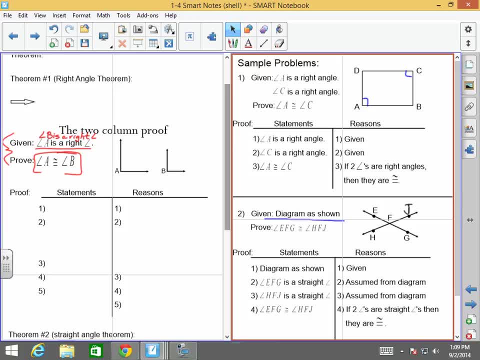 are straight angles, they're congruent. So theorems as much as of a nightmare it could be. my friends, it actually makes things easier Because we didn't have to define that the measure of these angles were 180.. We knew. 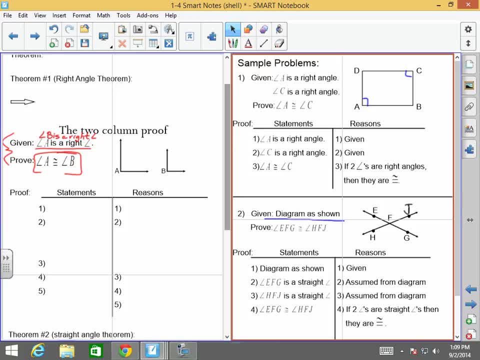 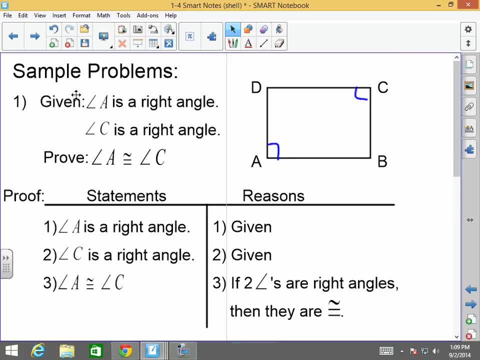 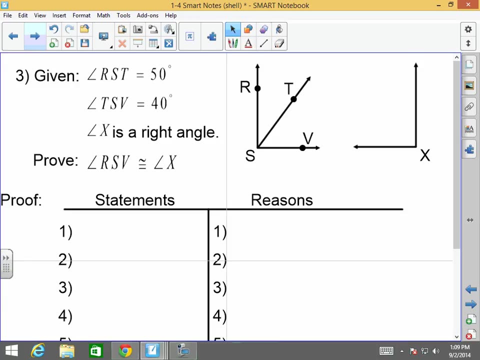 the theorem already: If they're both straight angles, they're congruent. Does that help guys? Alright, You guys are doing great. Thank you so much. Okay, So we did one and two. Okay, Let's do another one now. Okay, 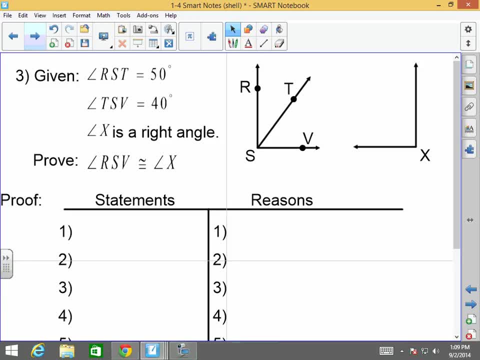 I have got here, given that angle RST is 50 degrees. Yes, sir, No, no, no, Go ahead. You were going to ask: Okay, let me just prep it up, and then you got it. Thank you, my man. Angle RST is 50 degrees. 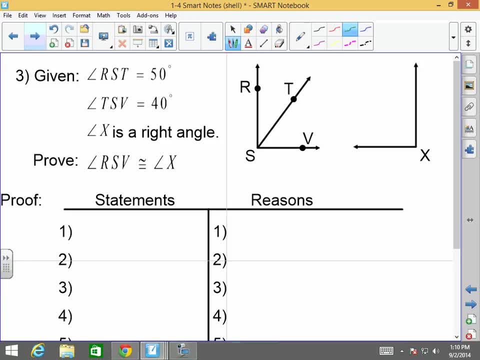 I'm a big, big, big, big, big believer in labeling Huge, So write it: RST is 50. Awesome. TSV is 40.. Cool beans: TSV is 40. Awesome. Angle X is the right angle. Alright, I know that's a right angle. 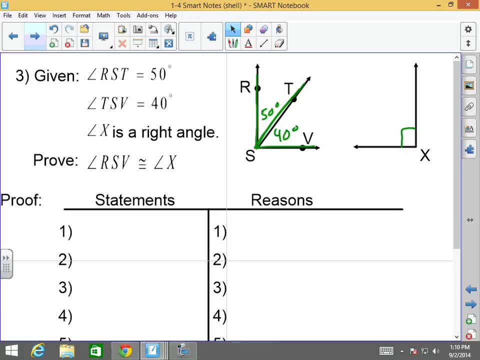 I've drawn it. Why do you draw it, Mauro? It says it right there. Why are you wasting your time? I'm not. I promise you, The more you mark up your figure, the more valuable information just kind of pops up to you. Okay, So what would you think? 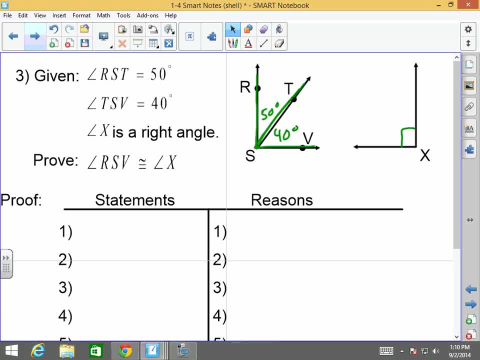 my first statement would be my brother: Yeah, Very good, RST equals 50 degrees. The measure of our angle, RST, is 50 degrees. Why, Awesome? What else, brother, Can I really go anywhere with that? Can that given give me more information? 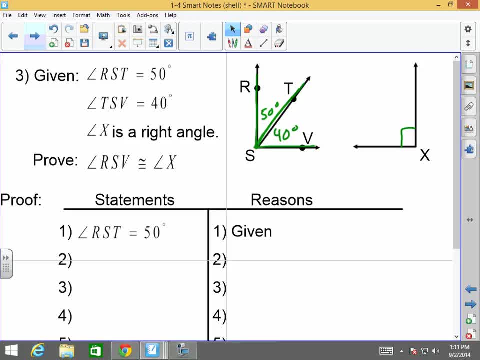 Really Okay. What can that give me Wrong? Thank you so much. He jumped a big, big step. He said: angle RST is 50 degrees. and then he wanted to say next: the sum of RST and TSV is 90. You haven't even defined what TSV is yet, brother. 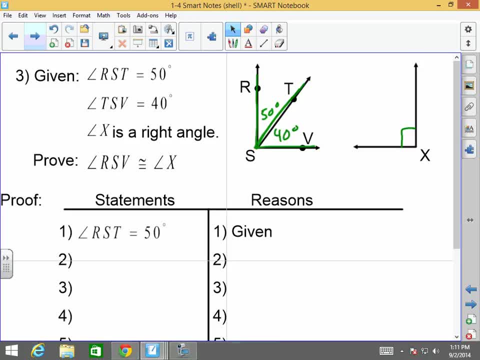 Okay, And remember, guys, this is a process You guys are doing great. So, that being said, what do you think step 2 would be here, gentlemen, Go ahead, Go ahead, Say it. Angle TSV is equal to 40 degrees. 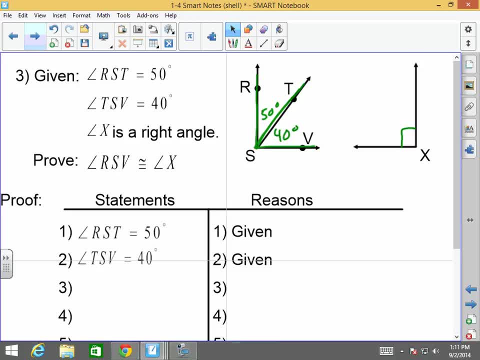 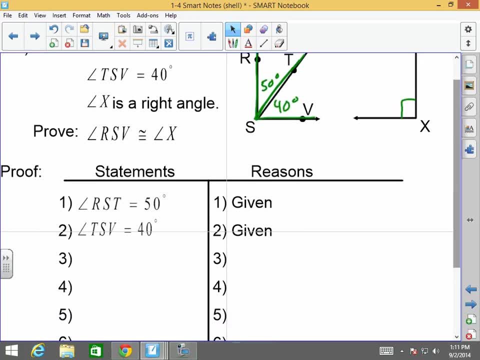 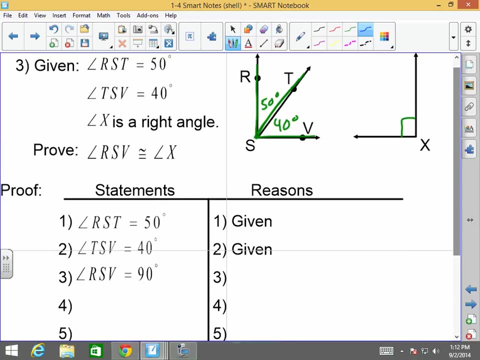 Why, Given Now, my brother, what were you going to say? Thank you very much, sir. So I kind of condensed that and I said: okay, since RST is 50 and TSV is 40, that means that RSV the whole. 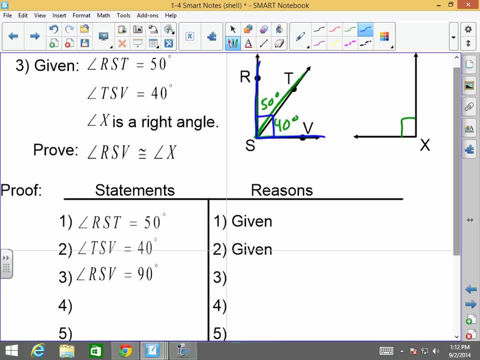 kit and caboodle is 90.. Why Simple? Think simple. Thank you. It's called the addition property. It's that simple. Keep it simple. silly, That's an engineering principle. It's called KISS. Alright, Keep it simple. 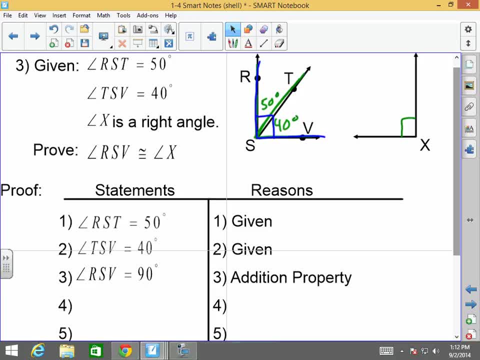 bro, Keep it simple. Addition property: 50 plus 40 is 90. So that means that if angle RST is 50 and TSV is 40, well heck, 50 plus 40 has to be 90. Why? Because we learned how to add a while ago. Addition property. 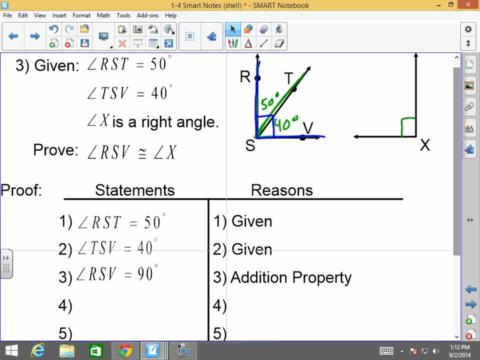 I'm not being sarcastic, It's that easy, Sir. You can't do the right angle theorem yet. Have you proven that that's a right angle yet Exactly, You guys are doing so great. Okay, you can't jump to right angle there. You first have 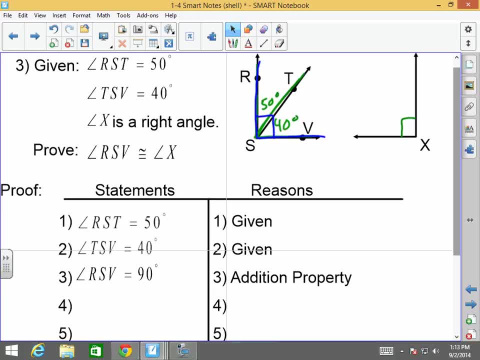 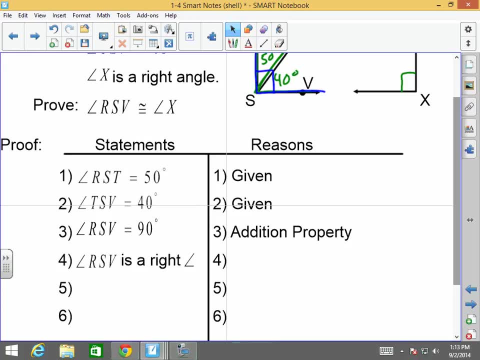 to prove that RSV is 90 degrees. Now that it's 90 degrees, what do we know? RSV is a right angle, is it not? Why, Okay, you can't say that's what a right angle equals? What's the? 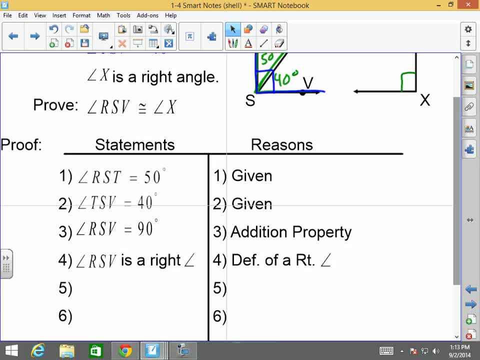 definition of a right angle. The definition of a right angle is that it equals 90 degrees. Yes, sir, Yes, technically we should have put M for the measure. Sorry, that's my bad. Thank you, sir. Okay, I'm not too much of a stickler for that, I'm not. 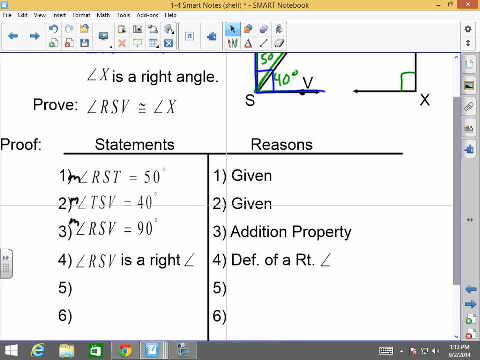 Just know that when you see that M, it means the measure. Okay, thank you so much for caring. You guys are great. Sir, You want to do 5?? Killer What you got, Love it. Angle X is a right angle, Y my brother, Heck. yeah, Now wait a second. 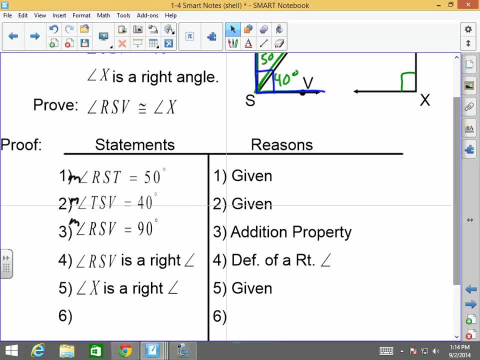 Something should be just kind of vibrating in your brain. What theorem do we know already? If they're both right angles, what do we know? How do we prove that RSV is congruent to angle X? Because No, not if they have. 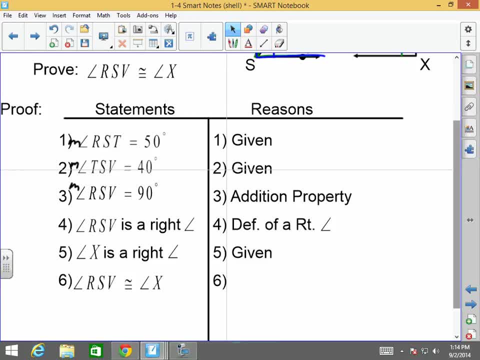 the same. No, not if they have the same measure. Thank you, if two angles are right angles, then they're congruent. Now to go back to what my boy said: We cannot use in this case: if two angles have the same measure, then they're congruent. 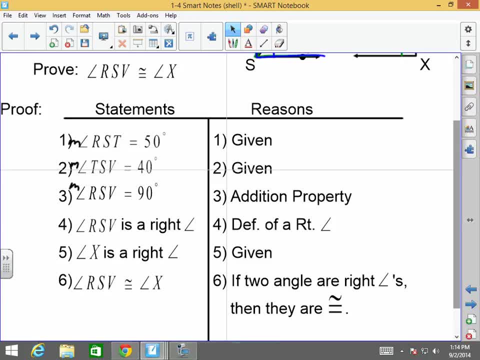 Did we define the measure of angle X or did we just define it being a right angle? Do you see where I'm going with this, guys? If I had said now, after the X is a right angle, the measure of angle X is 90 degrees, then you could. 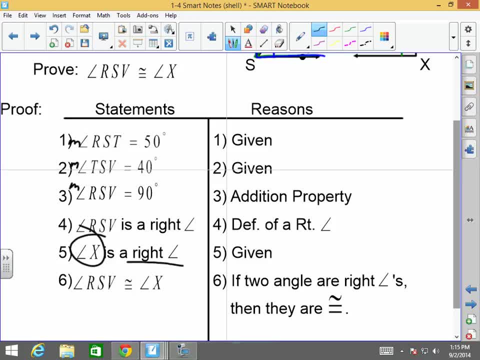 have said, if two angles have the same measure, then they're congruent. But we didn't define both angles as measures. We defined both angles as right. So keep it simple. Don't add extra steps if you don't have to. Sir. 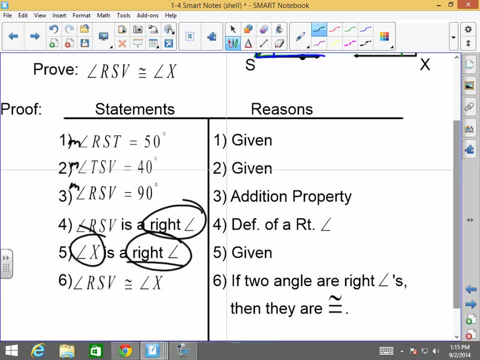 Okay, on a quiz or a test, can we add extra steps? Yes, But trust me, after you're doing a bunch of these, you're going to want to not add extra steps. But yes, you may, Sir. Yes, Okay, Great question. 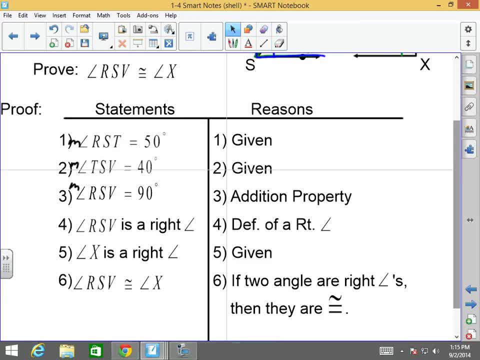 The question here is: Mr Morrow, for 4 and 5, couldn't I switch the order? Couldn't I put this one here and this one here? Yes, but be careful. The reason that I went in this direction, the reason I flowed this way, was because, didn't I? 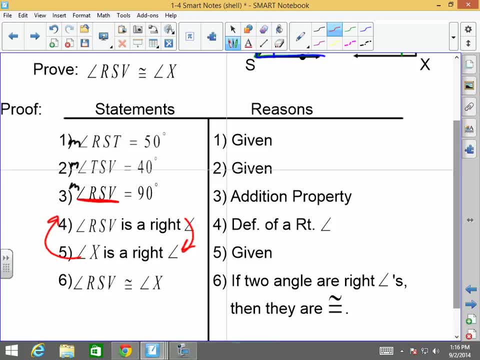 already prove that RSV was 90?? Let's stick with the information we have. If RSV is 90, that means RSV is a right angle. Now you can get to the X is a right angle and then you can prove it because you've proven that both are right angles. 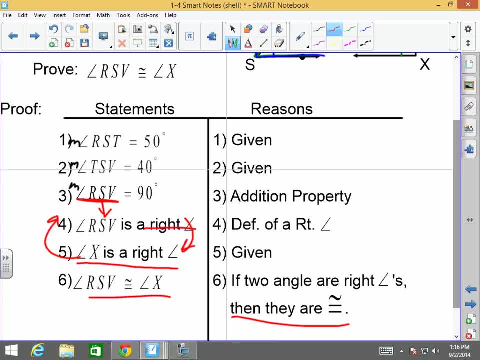 Is that making sense to you? Yeah, You sure, my man, But it can also be in 3, right, 5 could be in 3 as well. Yes again, yes, it can. Everyone is going to think a little differently. 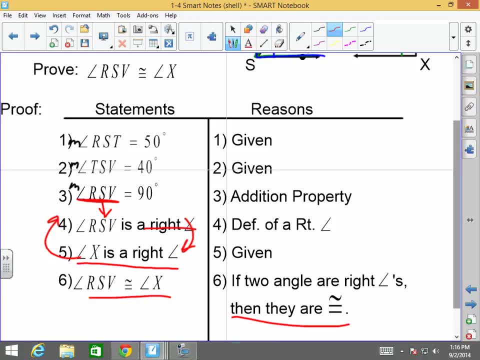 here. okay, As long as the facts are there, I'm not too worried about the order. but I don't want to train you a poor way. It's better to train you to show you. okay, go in sequence and show what each statement is giving you in a sequence. But the answer is yes. 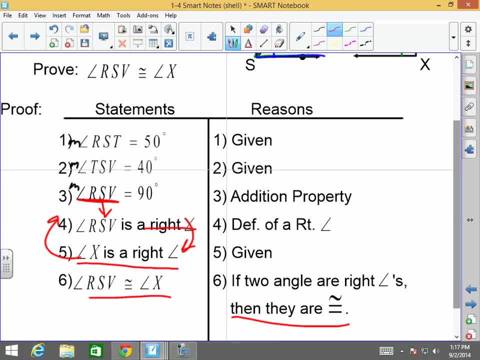 Sir. and then, sir, Yes, we had already, yes, Someone had asked that before. Could you write right angle theorem? Yes, you may, You are totally allowed. Thank you, Sir. Okay, Yes, okay. Now that's a great question. That is a no-no. What my boy. 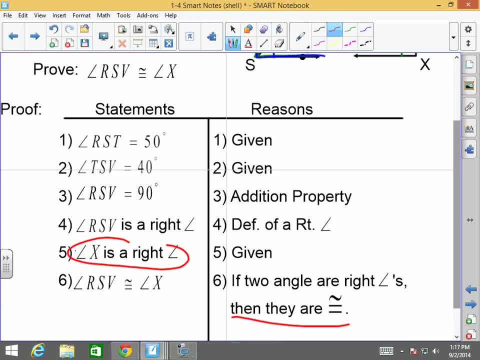 had asked before was Mauro, can I put this one here? Yeah, you can. It wouldn't make logical sense, though, But now, what you asked, sir, was very important and very dangerous. okay, He said, can I move this guy? 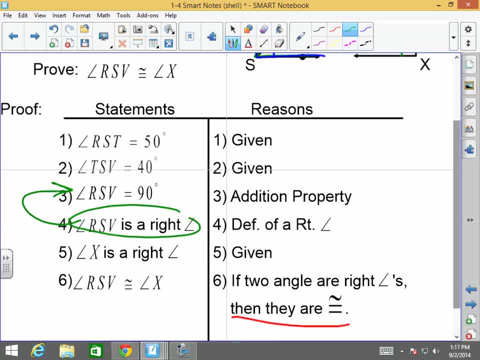 here. No, No, You cannot move that there, because you haven't proven yet that these two angles equal 90.. You can't have a right angle, my brother, unless you know it's 90 degrees, Correct, sir? You couldn't have definition. 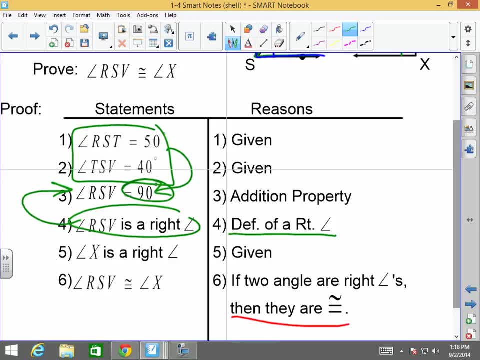 of right angle yet because you haven't defined that it's 90. So you couldn't switch three and four. no, Does that make sense? Does that make sense to everybody? Awesome, You guys are doing great today. Awesome, And. 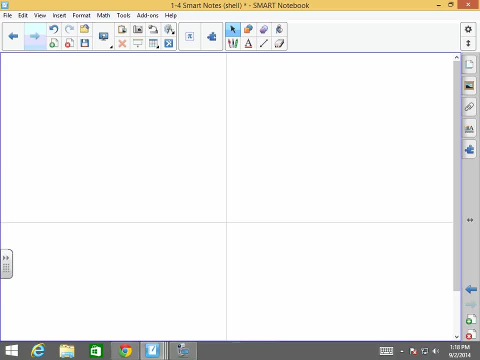 boom, we are done. I hope you learned a lot, guys. We're going to do some practice problems together now and thank you. 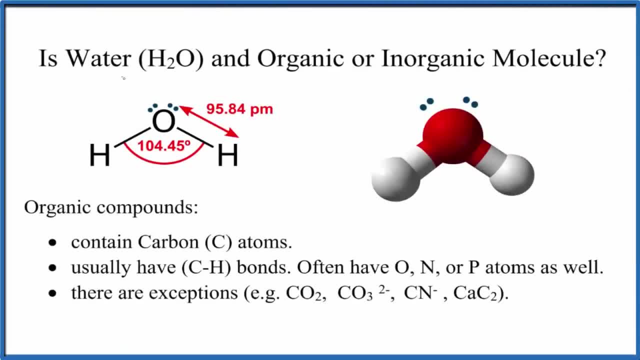 The question is whether water, H2O- is an organic or an inorganic molecule. So we have a general definition here. It says that organic compounds, they'll contain carbon. So right away we see H2O. We have two hydrogens and the one oxygens. There's no carbon there. So water is not an organic compound. We consider water an inorganic molecule. 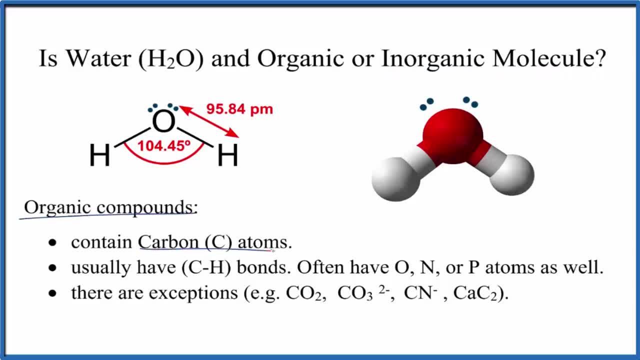 So with organic compounds. we said it contains carbon. Often it'll have hydrogen atoms too. It'll have carbons bonded to hydrogens. Sometimes it'll have oxygen, nitrogen and phosphorus atoms as well, And there are some exceptions like CO2, carbon dioxide is considered inorganic, So we've classified water as inorganic, but it does share something in common with organic compounds. Let's take a look at the periodic table. 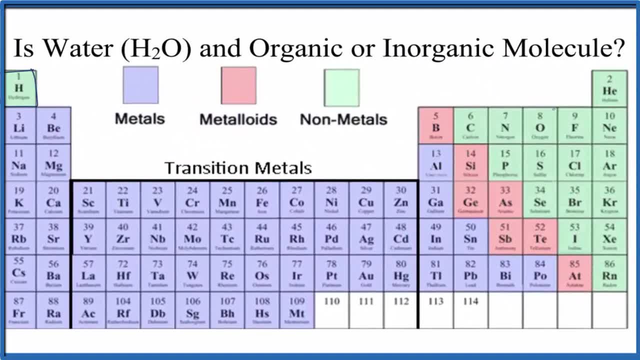 So if we find hydrogen here and oxygen, they're both inorganic, So we have both nonmetals. When we have two nonmetals we have a covalent compound, also called a molecular compound. With organic compounds we have carbon bonded to things like hydrogen or nitrogens or oxygens and some phosphorus atoms. These are all nonmetals. So water is a molecular compound. In organic compounds they're going to be molecular too. That means they have covalent bonds and the electrons are shared between the atoms. So even though water is considered an inorganic compound, it's not. 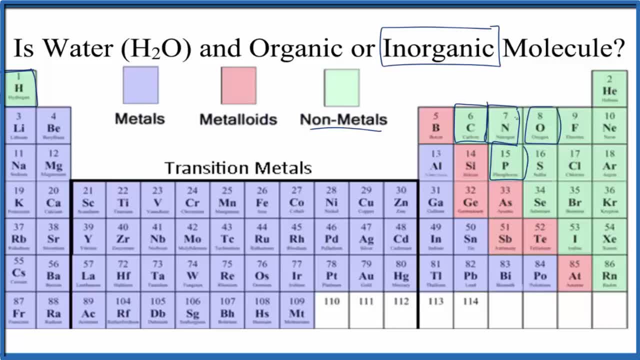 It does have covalent bonds in it, just like organic compounds do. This is Dr B answering the question whether water is an organic or inorganic molecule. It's inorganic because it doesn't contain carbon. Thanks for watching.